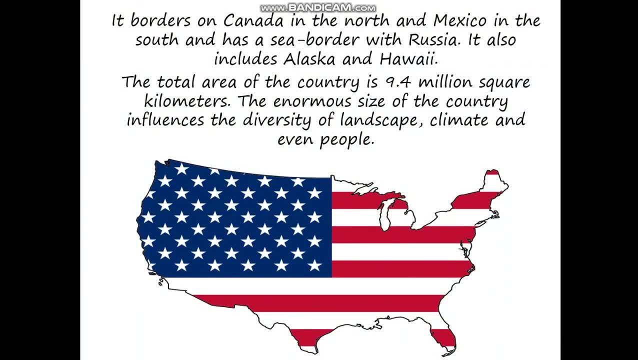 It borders on Canada in the north and Mexico in the south, and has a sea border with Russia. It also includes Alaska and Hawaii. The total area of the country is 9 million square kilometers. The enormous size of the country influences the diversity of landscape, climate and even people. 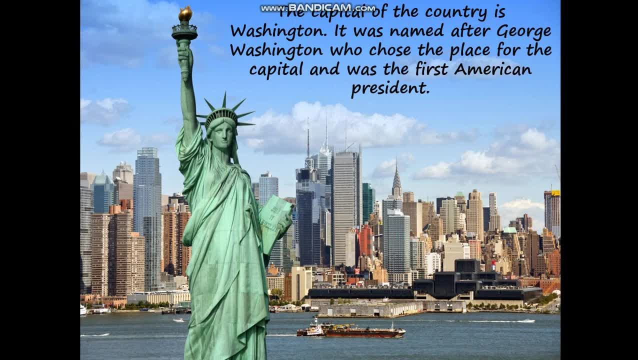 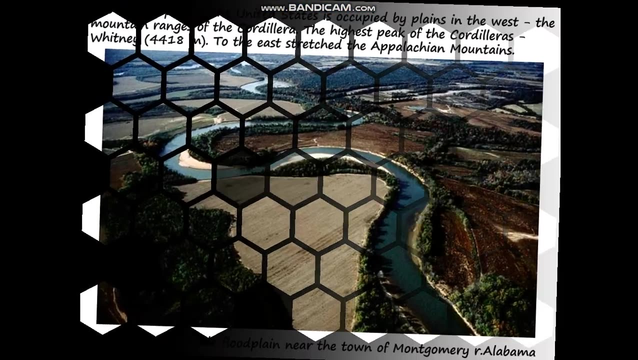 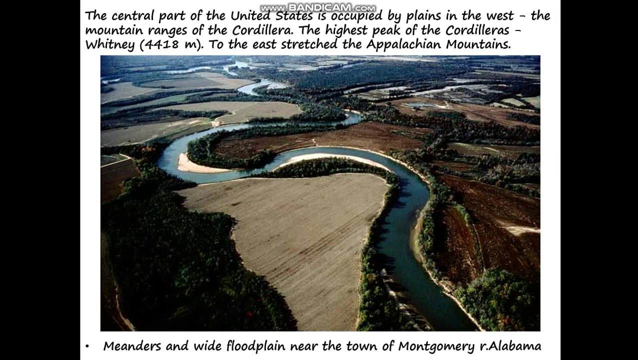 The capital of the country is Washington. Washington was named after George Washington, who chose the place for the capital and was the first American president. The central part of the United States is occupied by plains, In the west, the mountain ranges of the Cordillera, the highest peak of the Calderilla Whitney. 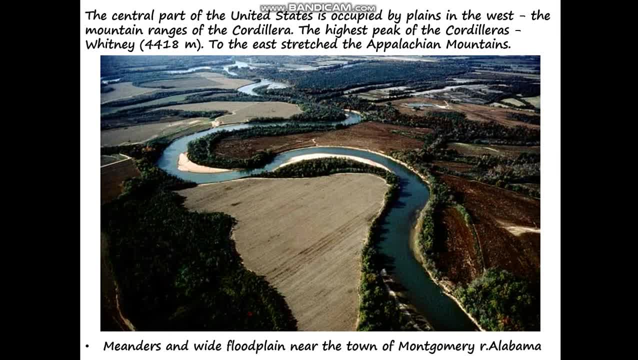 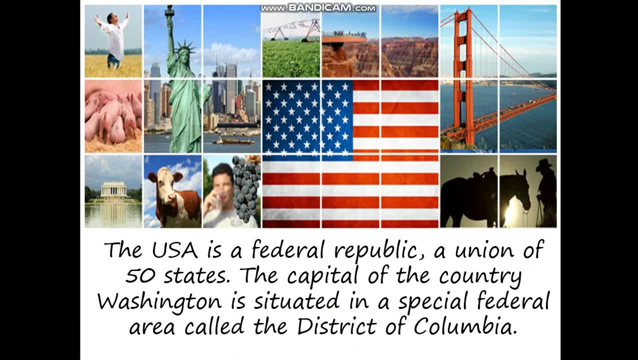 To the east stretch, the Appalachian Mountains. To the west stretch, the Appalachian Mountains. The USA is a federal republic, a union of 50 states. The capital of the country, Washington, is situated in a special federal area called the District of Columbia. 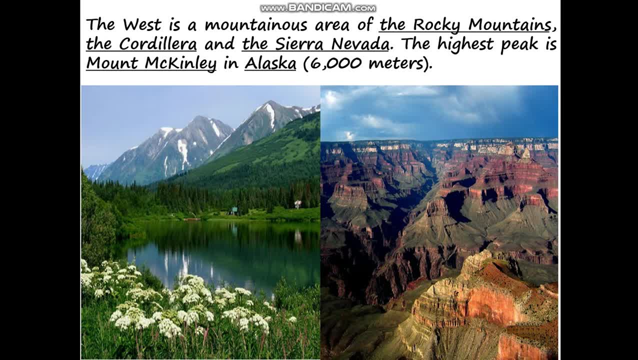 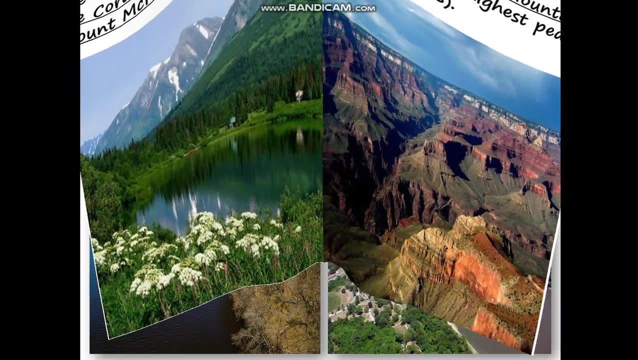 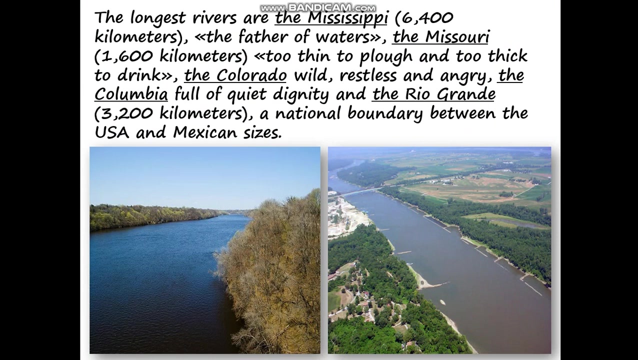 The west is a mountainous area of the Rocky Mountains, the Cordillera and the Sierra Nevada. The highest peak is Mount McKinley in Alaska. The west is a mountainous area of the Kansas River. The longest rivers are the Mississippi, the Father of Waters, the Missouri, too thin to plough and too thick to drink. 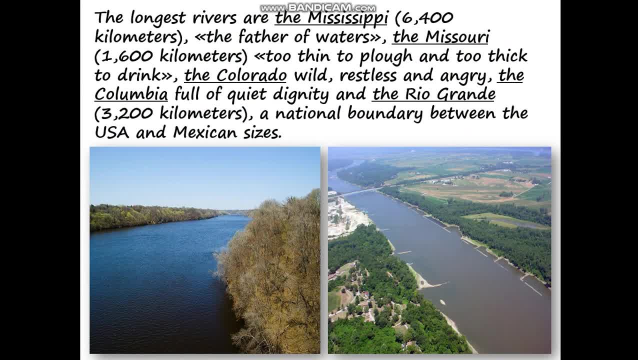 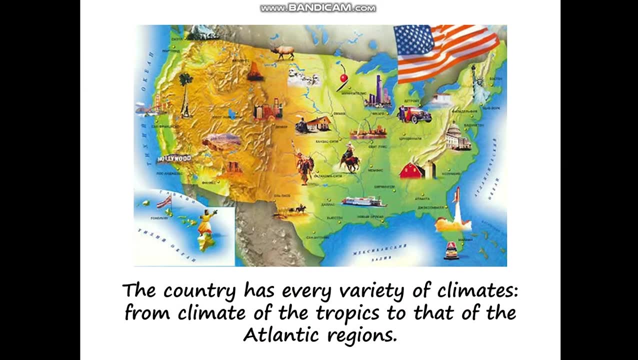 The Colorado Wild, restless and angry. The Columbia full of quiet dignity, And the Rio Grande a national boundary between the USA and Mexican sizes. The country has every variety of climates, from climate of the tropics to that of the Atlantic regions. 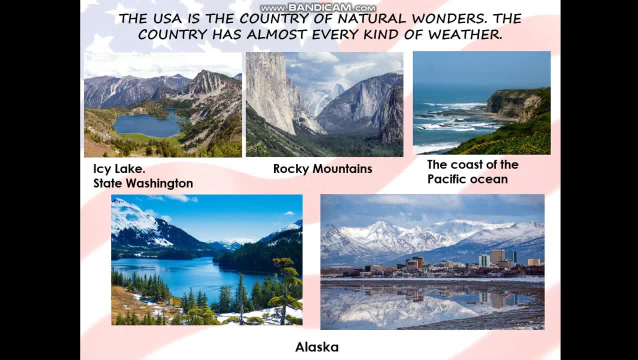 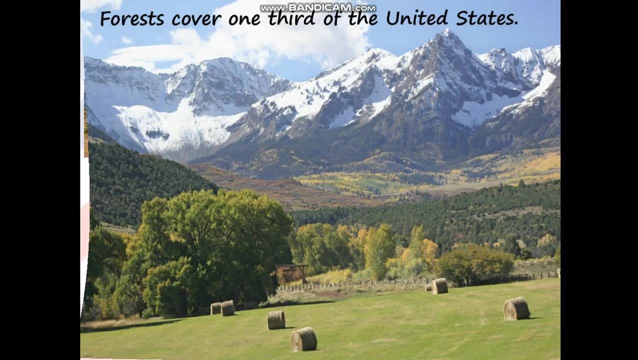 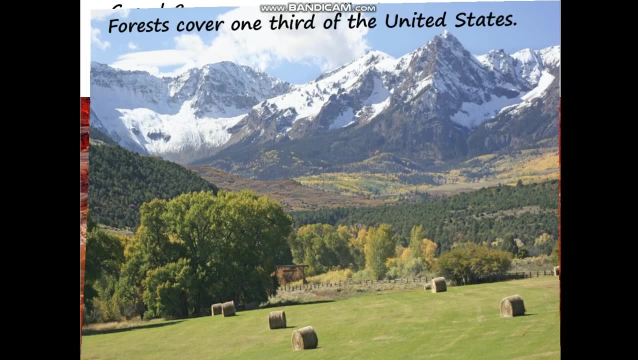 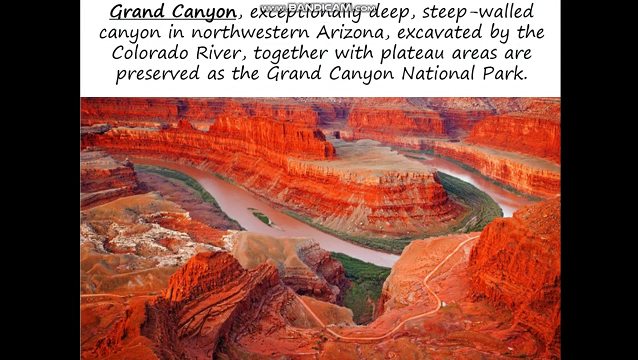 The USA is a country of natural wonders. the country has almost every kind of weather. Forests cover one-third of the United States. Grand Canyon, exceptionally deep, steep-walled canyon in northwestern Arizona excavated by the Colorado River, together with plateau areas, are preserved as the Grand Canyon National Park. 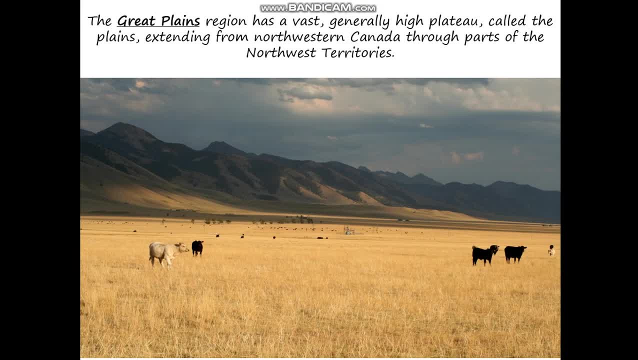 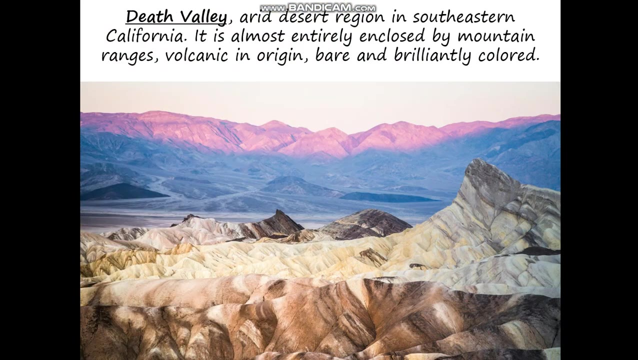 The Great Plains region has a population of over 1,000,000.. It has a vast, generally high plateau called the Plains, extending from northwestern Canada through parts of the Northwest Territories, Death Valley, arid desert region in southeastern California. 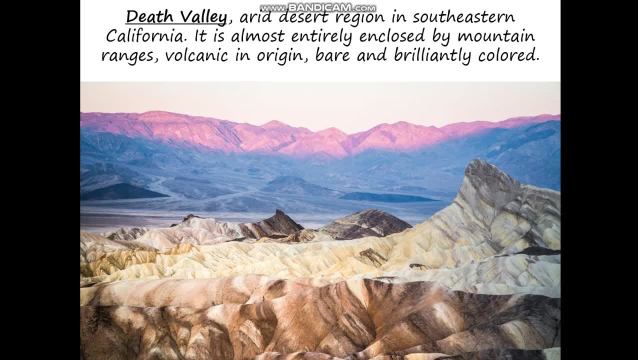 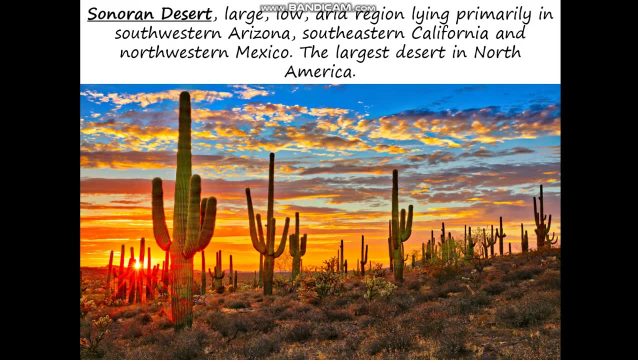 It's almost entirely enclosed by mountain ranges, volcanic in origin, bare and brilliantly colored Sonoran Desert, large low arid region lying primarily in the middle of the desert. It is a large desert in southwestern Arizona, southeastern California and northwestern Mexico. 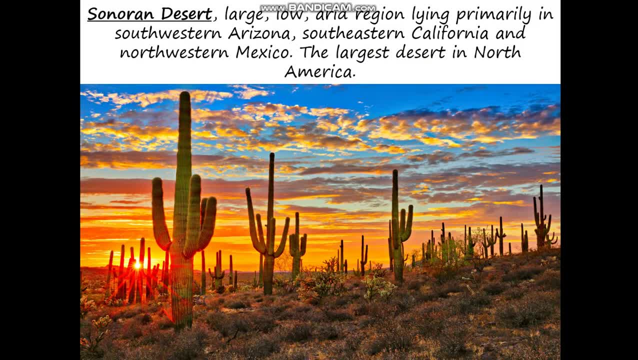 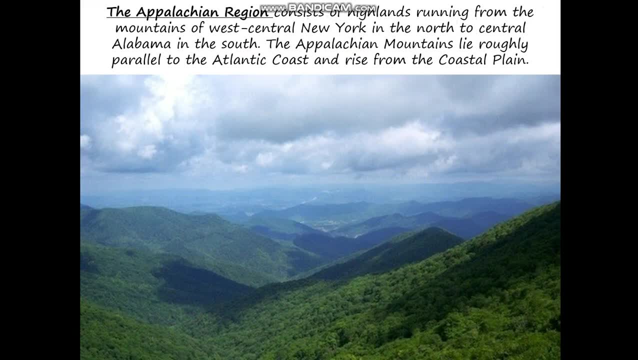 The largest desert in North America. The Appalachian region consists of highlands running from the mountains of west-central New York in the north to central Alabama in the south. The Appalachian Mountains lie roughly parallel to the Atlantic coast and rise from the coastal plain. 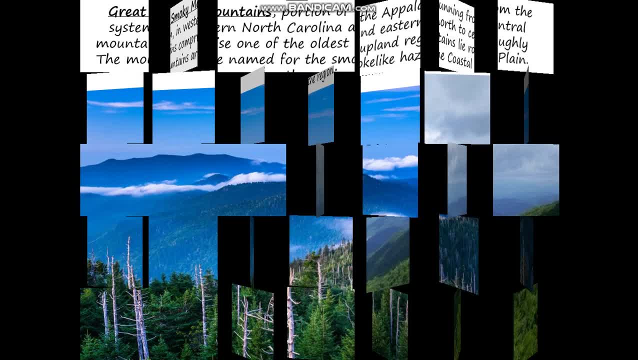 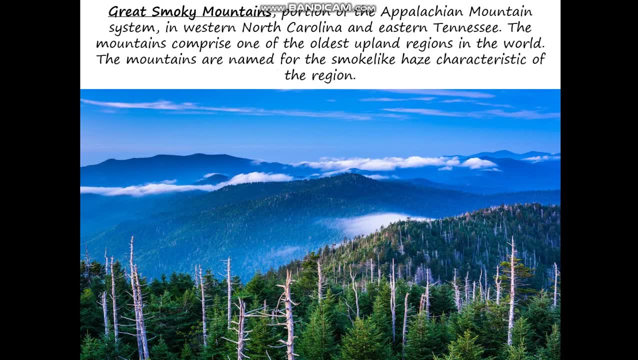 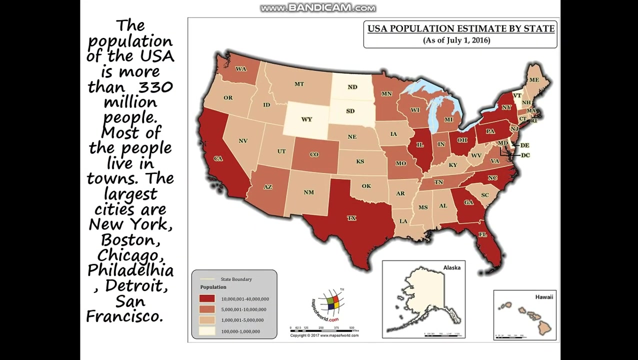 The Appalachian Mountains lie roughly parallel to the Atlantic coast and rise from the coastal plain Great Smoky Mountains, Portions of the Appalachian mountain system in western North Carolina, Alaska and eastern Tennessee. The population of the USA is more than 330 million people. 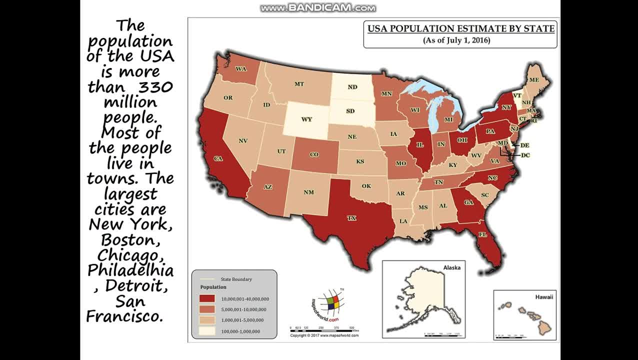 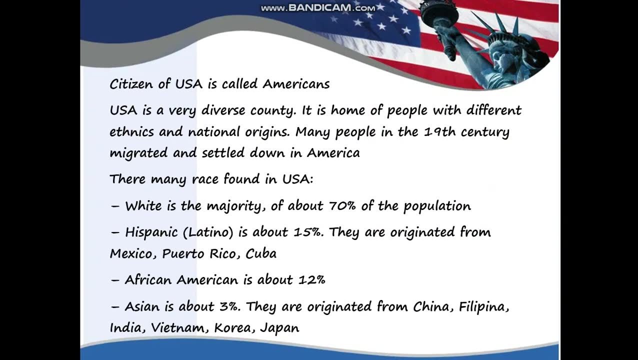 Most of the people live in towns. The largest cities are near the geological horizon. Theativas are very timber. Largest cities are New York, Boston, Chicago, Philadelphia, Detroit, San Francisco. Citizen of the USA is called Americans. USA is a very diverse country. 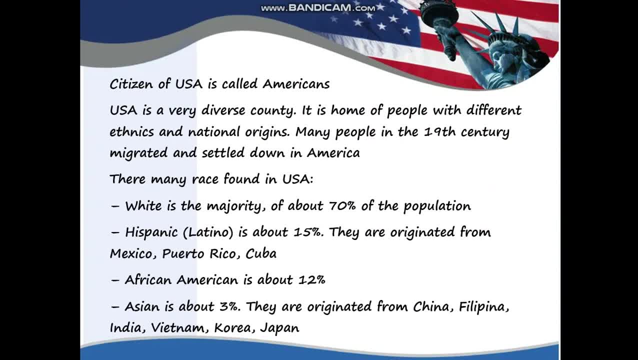 It's home of people with different ethnics and national origins. Many people in the 19th century immigrated and settled down in America. There are many races found in USA. White is the majority of about 70% of the population. Hyphenic Latino is about 15%. 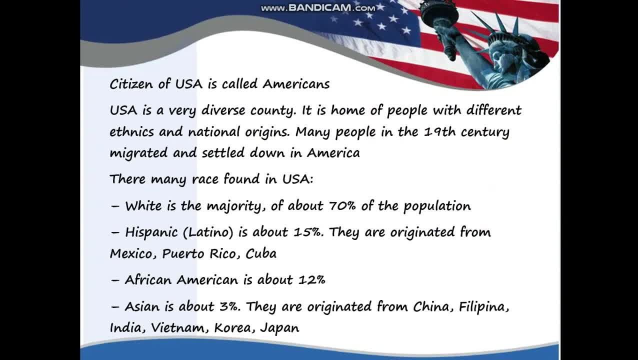 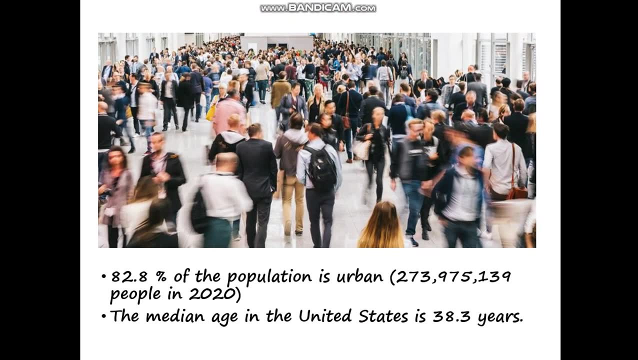 They originated from Mexico, Puerto Rico, Cuba. African American is about 12%, Asian is about 3%. They originated from China, Filipina, India, Vietnam, Korea, Japan. 82.8% of the population is urban. The median age in the United States is 38 years. 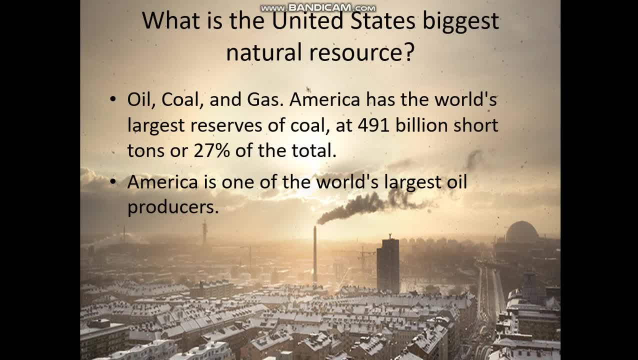 What is the United States' biggest natural resource? Oil, coal and gas. America has the world's largest reserves of coal at 491 billion short tons, or 27% of the total. America is one of the world's largest oil producers. 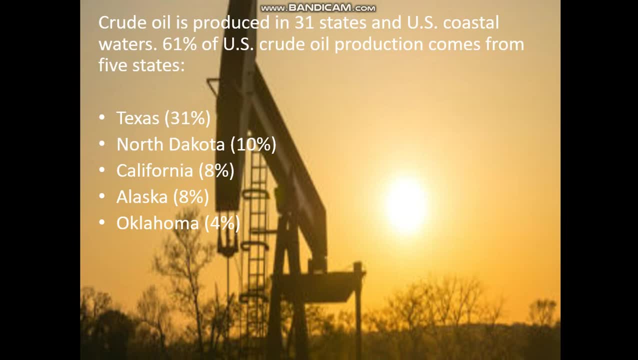 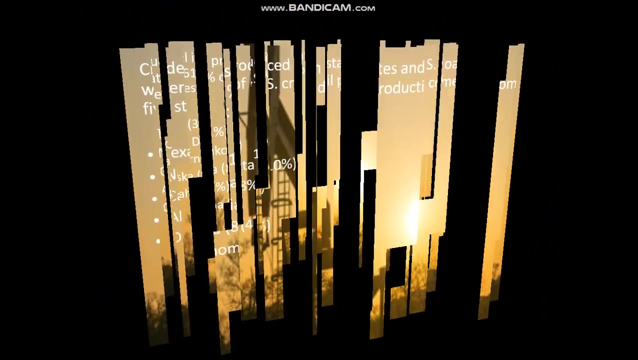 Crude oil. Crude oil is produced in 31 states and US coastal waters. 61% of US crude oil production comes from 5 states: Texas, North Dakota, California, Alaska, Oklahoma. The country is rich in mineral resources. 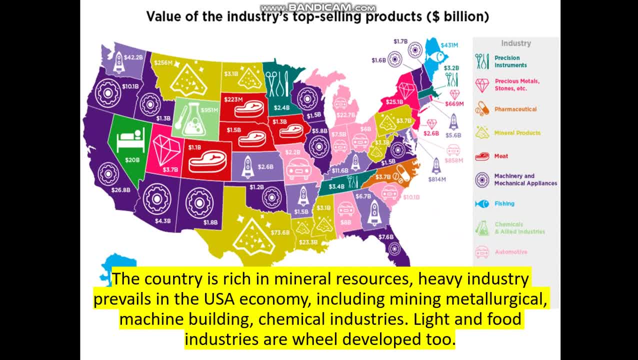 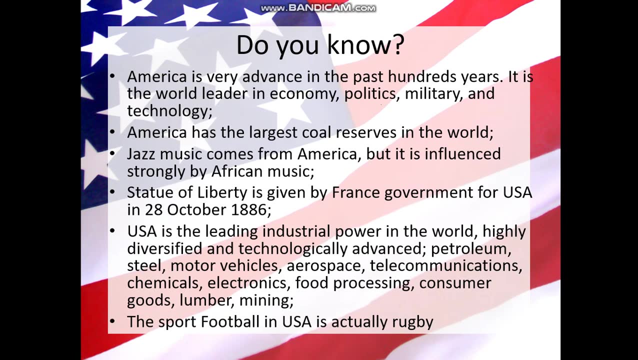 Heavy industry prevails in the USA economy, including mining, metallurgical, machine building, chemical industries. Light food industries are a field we'll develop too. Do you know that America is very advanced in the past 100 years? It's the world's largest leader in economy, politics, military and technology. 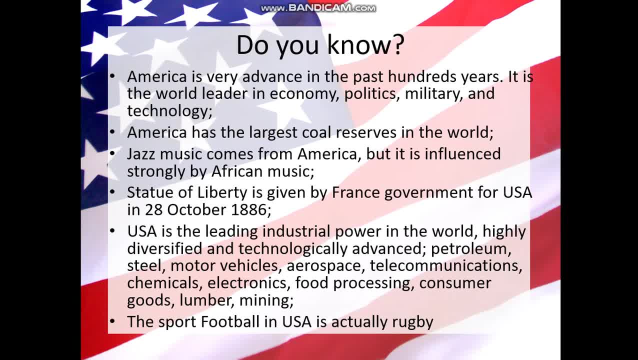 America has the largest coal reserves in the world. Jazz music comes from America, But it's influenced strongly by African music. The Statue of Liberty is given by the French government for the USA on October 28, 1886.. The USA is the leading industrial power in the world, highly diversified and technologically advanced. 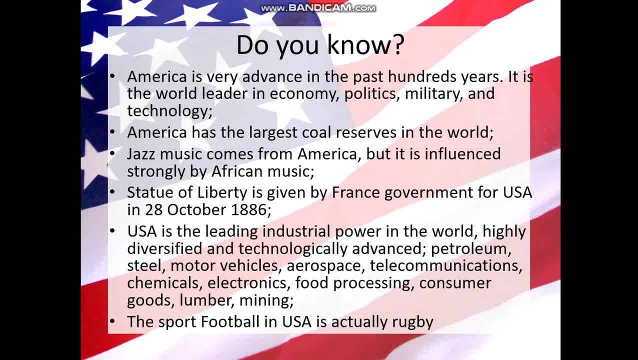 Petroleum, steel, motor vehicles, aerospace, telecommunications, chemicals, electronics, food processing, consumer goods, lumber mining. The sport football in the USA is the most popular sport in the world. The sport football in the USA is the most popular sport in the world. 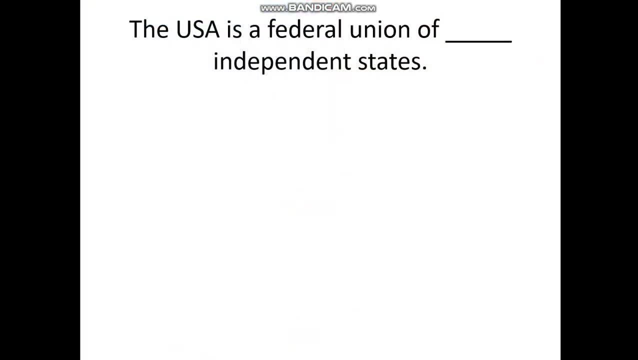 The sport football in the USA is the most popular sport in the world. The USA is actually a rugby. And now I have some questions for you. The USA is the federal union of independent states. How many states are there? The most recent state to join the union was